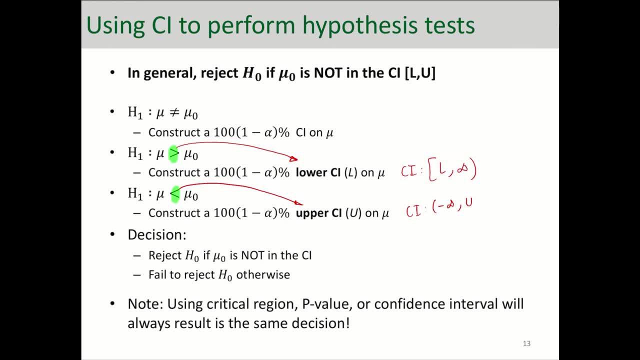 negative infinity all the way to an upper confidence limit. Okay, And this is how you make a decision: You would reject your null hypothesis if mu naught is not in the confidence interval. So this mu naught is something that you would have to check against the confidence interval. 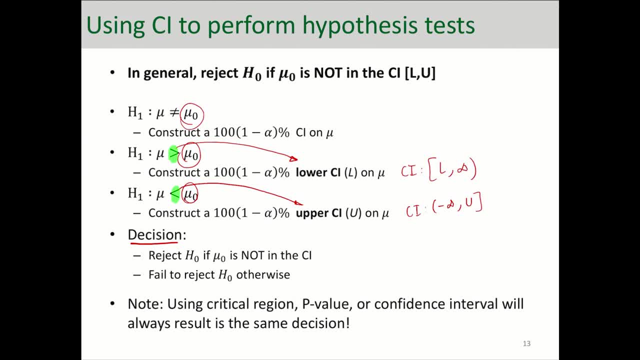 and you make a decision For a two-sided confidence interval. you would have a confidence interval with a lower limit, an upper limit. If the mu naught is not in the confidence interval, you reject the null hypothesis. Otherwise you fail to reject. 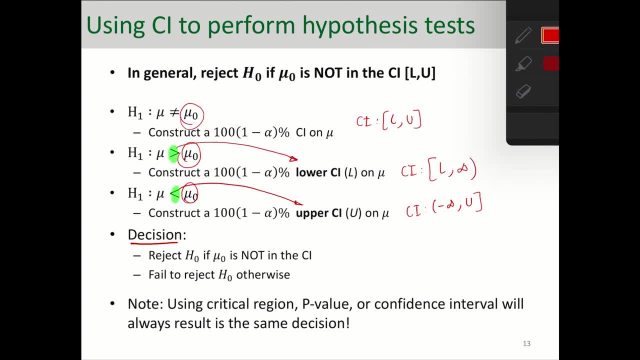 A very important point here is that in hypothesis testing we have these three methods of making decisions. We have critical region, We have p-value, We have confidence interval. It is very important here to remember that these three methods will result in the same decision. 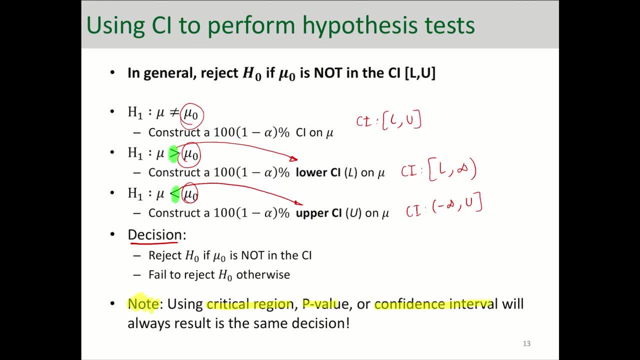 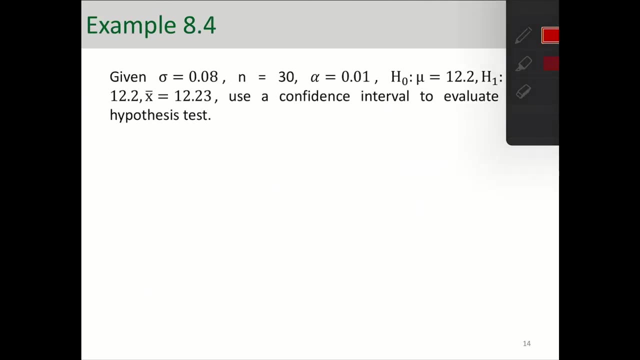 These are just different ways of making a conclusion about a hypothesis test, And all three of them will give you the same conclusion. It's just different ways of conducting the hypothesis test. So let's look at one example here that we had before. This is the example of volume of bottles. 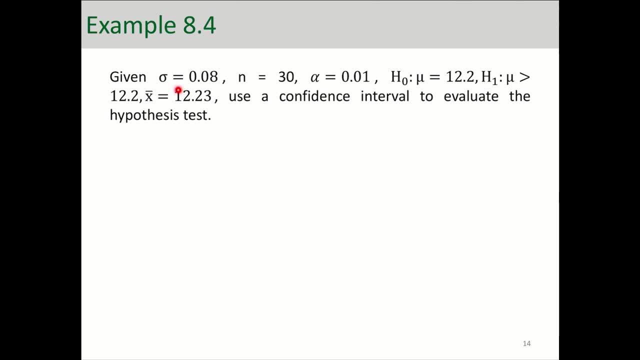 Basically, a company is making bottles And they want to make sure that the volume of these bottles is equal to 12.2 and- alternative hypothesis mu- more than 12.2.. They don't want to produce bottles that have a volume of more than 12.2 ounces. 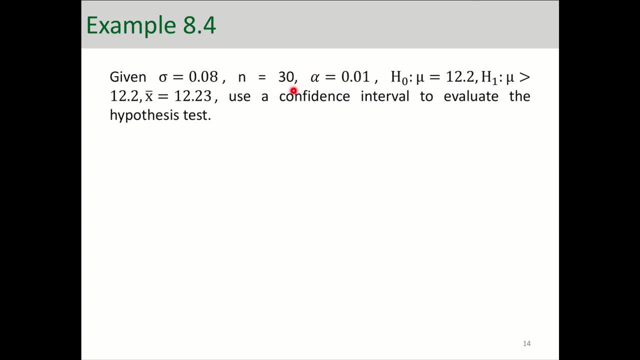 So what we do is we collect a sample of 30 bottles and we take the average volume of them- that's 12.23, with the alpha of 1%, use a confidence interval to evaluate the hypothesis test. So here we have everything that we need about a hypothesis test. 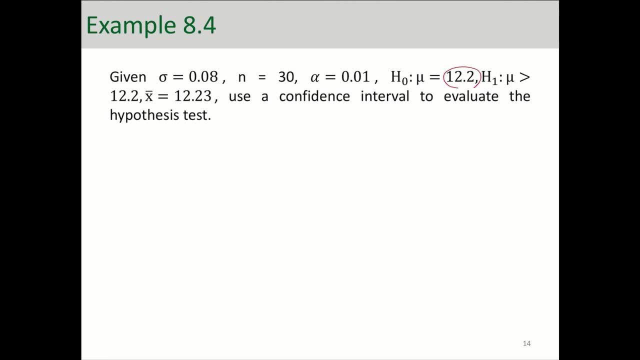 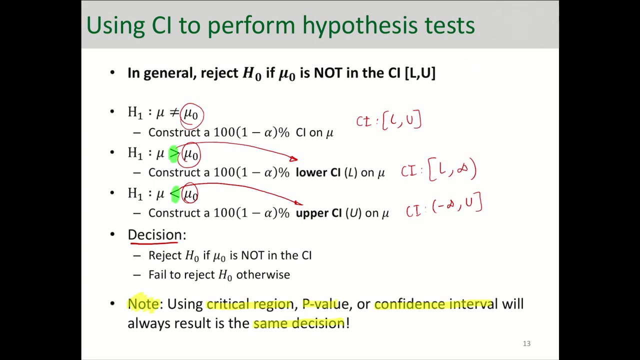 First, we know that our mu naught and we also know that our test is a one-sided test, one-sided hypothesis test, And with those two, we're basically looking at a confidence interval of this type, Because, Because our hypothesis test is one-sided with more than a sign, 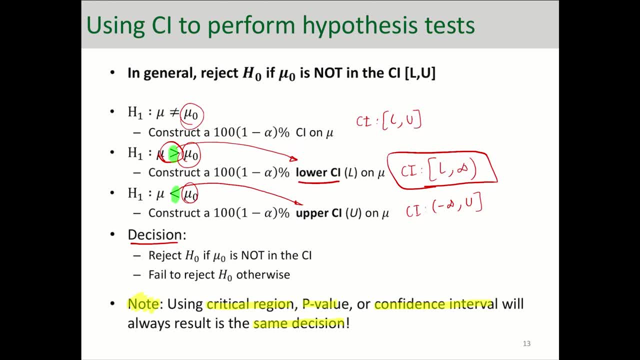 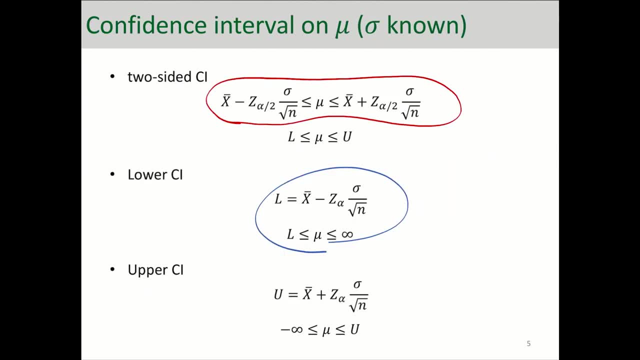 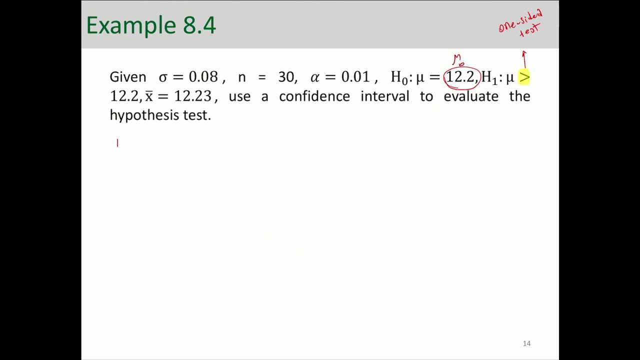 So we need to calculate the lower confidence limit. And how do we calculate the lower confidence limit? If I go back a few slides? here is the lower confidence limit: x, bar minus z of alpha times, sigma over square root of n. So I'll be calculating that. 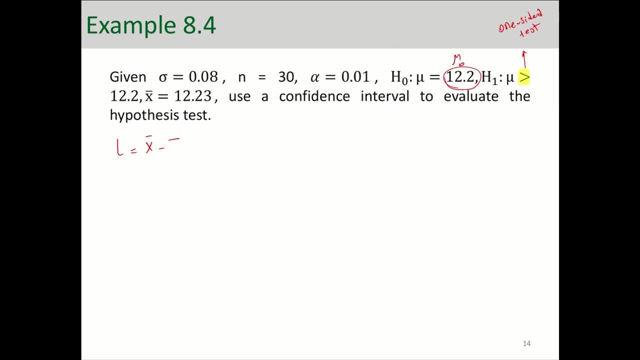 L or lower confidence limit is x bar minus z of alpha sigma, square root of n 12.23.. That's our sample average Minus z of 0.01 times 0.08 ounces over square root of 30.. 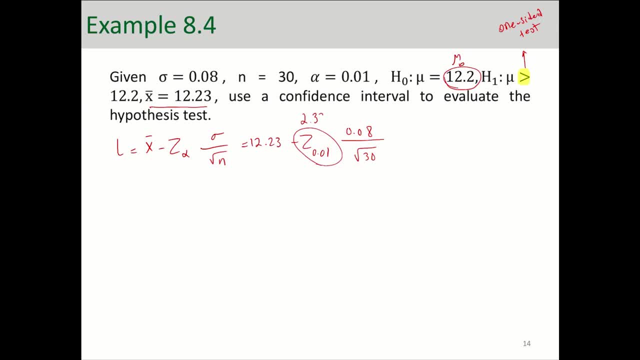 And this z value is 2.32.. You can read it from the normal z table And when you do the math here, That is equal to 12.196.. And that is the lower confidence limit. Basically, since our alpha is 0.01,, the confidence interval that we have here is a 99% confidence interval. that is, starting at 12.196 goes to infinity. 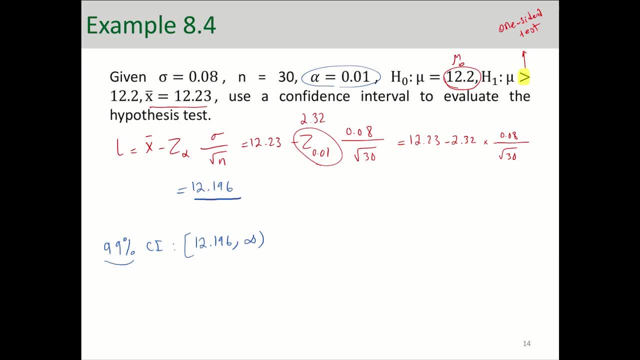 That's a one-sided confidence interval. It is 99% confidence interval, because that is 1 minus alpha. And what does this mean, This confidence interval? what does that mean? This means that, with 99% probability, the average volume of bottles is greater than 12.196..